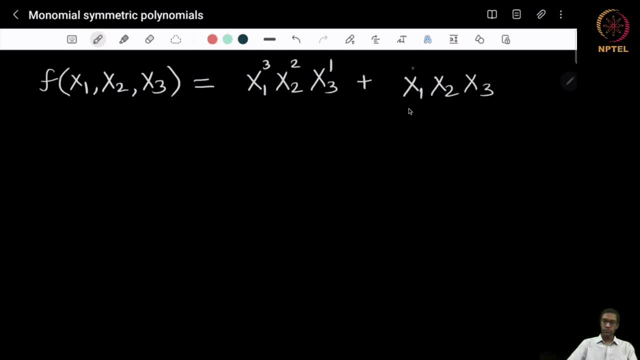 So I will just write, maybe one of them 3, 1, 2, maybe another 3, 2, 1, say 2, 1, 3, etcetera plus. So how does one think about what did we just do here? We started out with this basic monomial. Now any one monomial really, in this case. 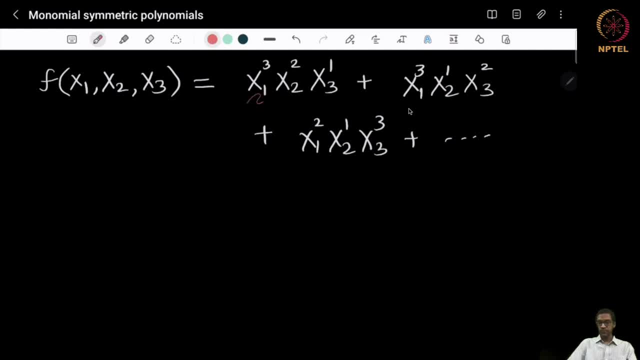 with a respect to x1,, x2, x3, with powers 3,, 2 and 3. And what we did is to sort of symmetrize it, add to this particular monomial all symmetrizations of that. So that was one example. 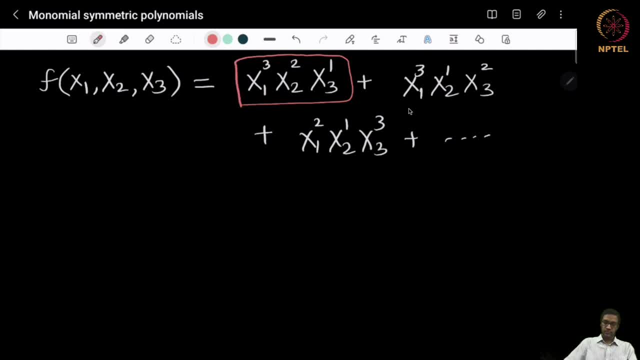 Now here is another one, So you could take the powers, say 4, 1, 1 plus all symmetrizations. ok, Now observe that. well, what are the symmetrizations here? you can put the 4 here, or I can put: 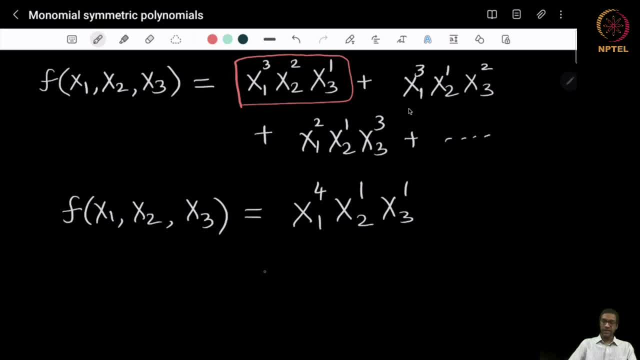 the 4 there. In this case I do not get 6 terms like I did in the previous one. I only get 3 of them. ok, So I started with this term and then symmetrized it. ok, but of course in this case I only get. 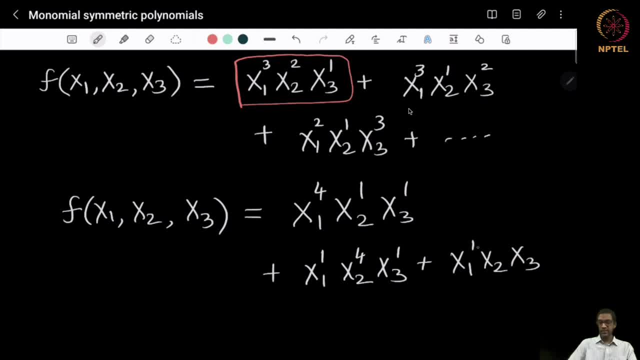 3 terms, and the reason I only get 3 rather than 6 is because there are 2 of these numbers are the same. ok, So I have 1 and 1 and because of that, what I have are only 3 terms. 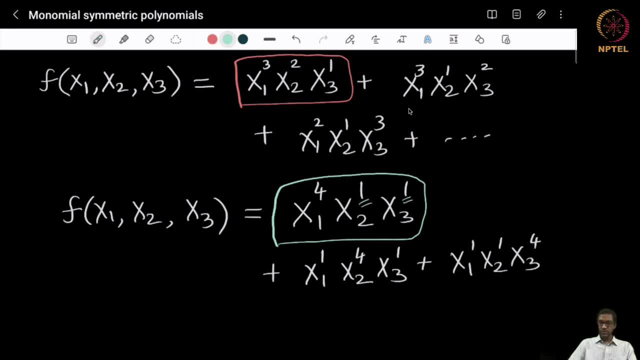 So these are both examples of what we will call monomial symmetric functions. So what is the? what is the basic definition? you start with a certain monomial. Now, I could have started with any of these in the earlier case, for example, any one of 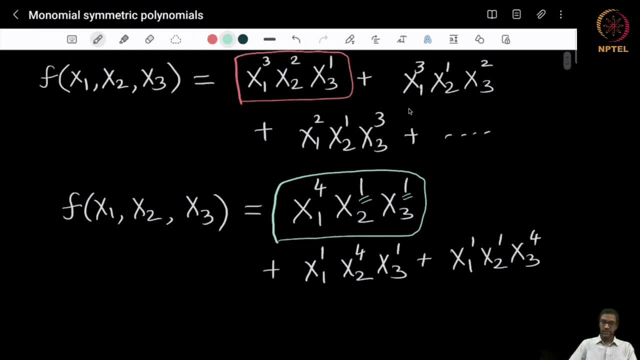 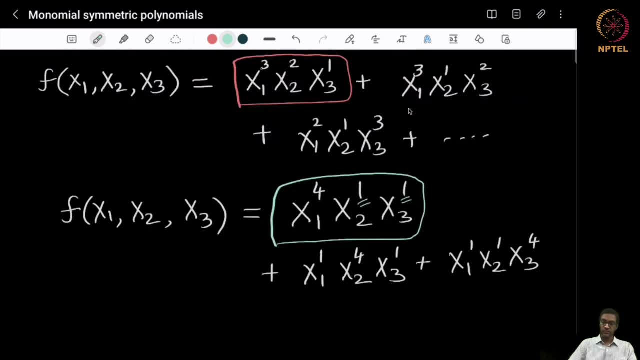 the 6 monomials and then symmetrized, but it is sort of more convenient to start with maybe a specific, a specific monomial. So the basic definition that we use is the following: that we always say, ok, let us start. 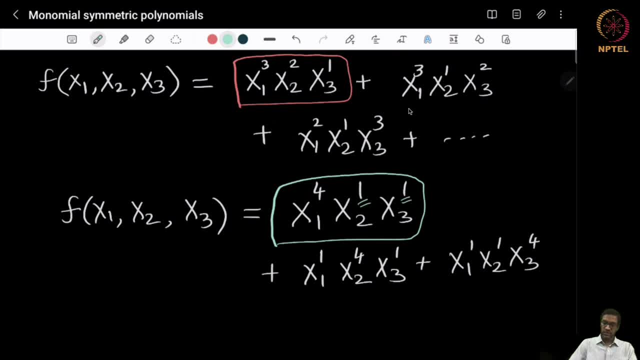 with this monomial whose powers are decreasing. So I have 3,, 2, 1, ok, So among these 6 monomials, there is one, exactly one, in which the powers are decreasing. right, because the others, the powers, are just obtained by permuting these numbers. and in the other, 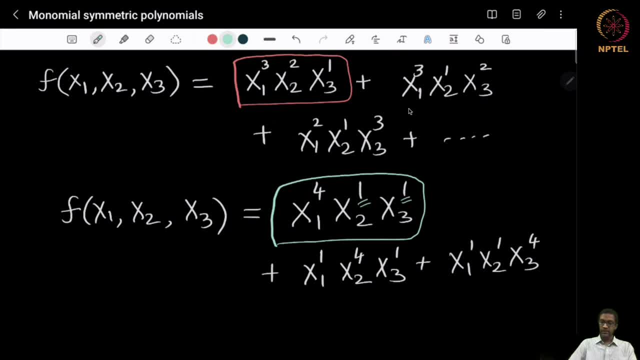 case. well, decreasing may not always work If you might only have weekly decreases. so 4, 1, 1 is a weekly decreasing sequence. So that is. that is something that that I picked. So let us give the general definition now. 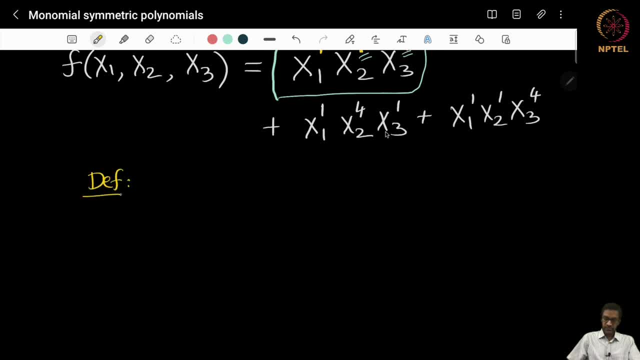 So given a Multi index, So let me just say definition. So let alpha be a multi-index, define lambda of alpha, So sometimes denoted. so let me give it two different notations. one is alpha, in decreasing. 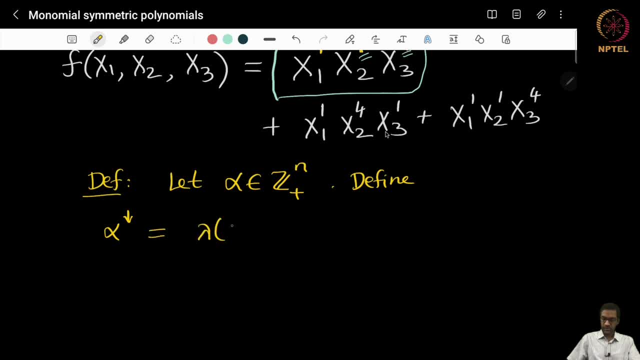 order, also denoted lambda, of alpha. So these are both two different notations. So here is the definition. This is nothing but the sequence, the sequence alpha 1 through alpha n, arranged in descending order. So the sequence of alpha i: i going from 1 to n, but rearranged in descending order. 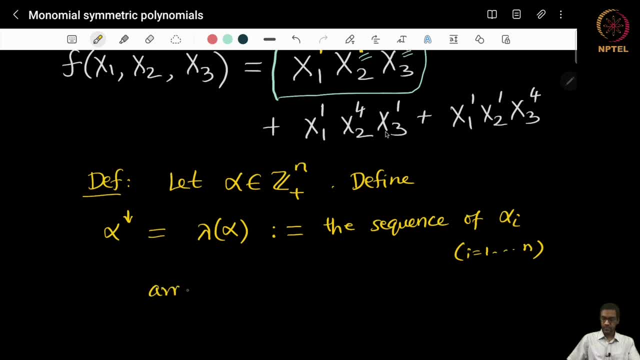 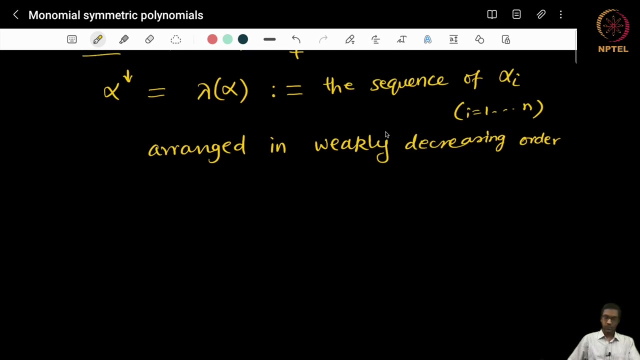 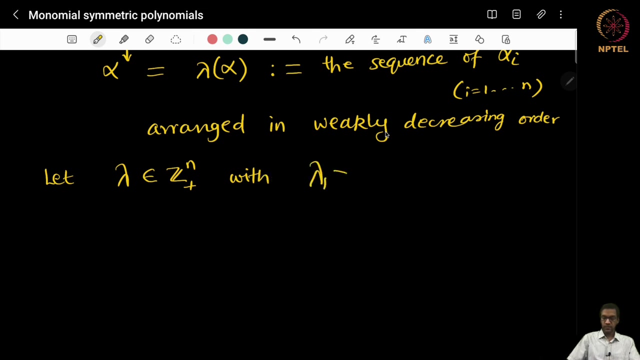 the sequence alpha. i arranged in weakly decreasing order, so that is just notation lambda of alpha. Now, given an element like this in weakly decreasing order, so let lambda denote a multi-index. let lambda be a multi-index, which is in weakly decreasing order, so it is z plus n that. 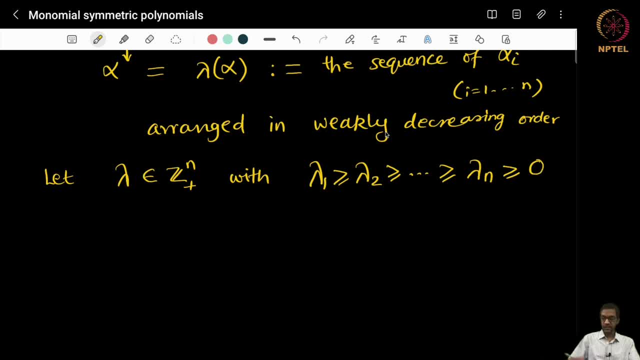 therefore, of course, all the lambda n's are positive, so I am just reiterating that fact. Now, given this, let us define. so here comes the main definition now- the monomial symmetric function or the monomial symmetric polynomial, called m sub lambda index by lambda of x: 1,. 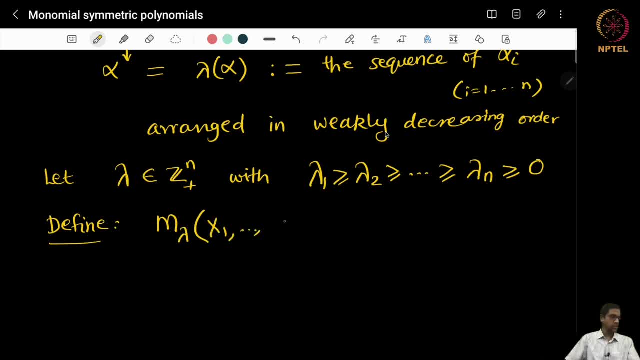 x 2, x n, the variables. This is defined as follows: you take the monomial x to the lambda. it is exactly like in the earlier two examples that we talked about. You take this one single monomial x to the lambda, then you symmetrize it in all possible. 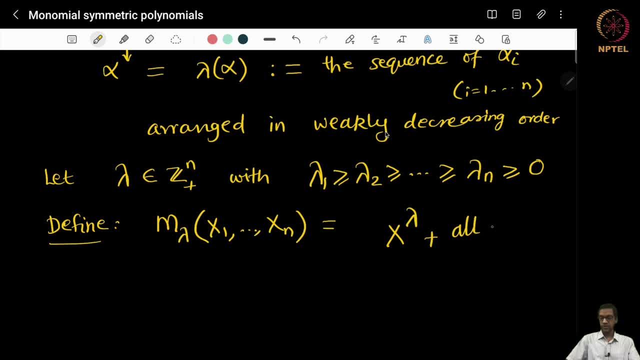 ways. plus- let me just write it informally for a start- plus all its symmetrizations. Now what does that mean? Let us write it out a bit more formally. This is: m. lambda is defined to be the sum of all monomial x to the lambda. 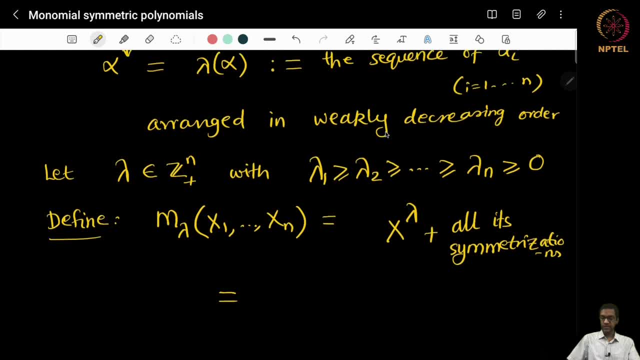 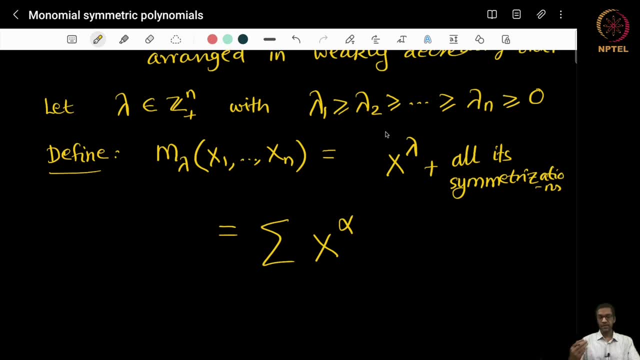 Now what does that mean? Let us write it out a bit more formally. This is m lambda is defined to be the sum of all monomial x to the alpha. Where, so how do you capture the statement that the multi-index alpha is the symmetrization? 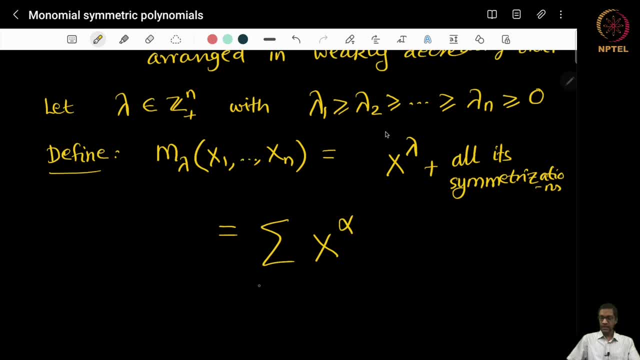 of the multi-index lambda. Well, if you rewrite alpha in descending order, so that is recall the notation we defined: lambda of alpha or alpha decreasing. so lambda of alpha should give you the original lambda that we fixed. So this is the definition, if you wish. 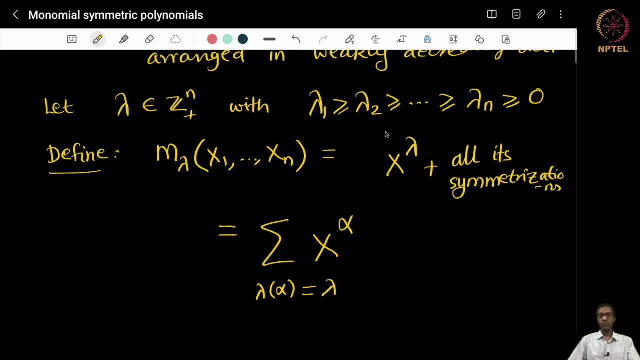 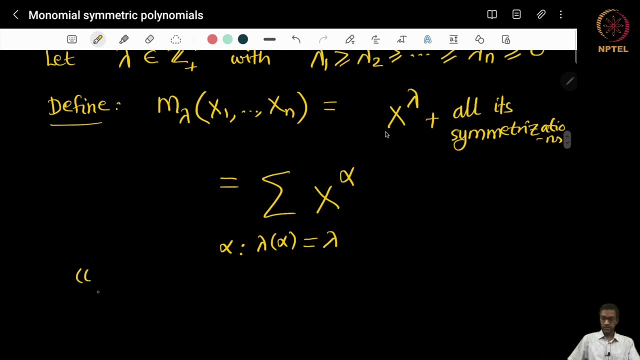 m, lambda of x, 1,, x, 2,, x n. So this is the definition, if you wish, the sum of all monomials, x to the alpha, where alpha ranges over alpha, such that alpha ranging over multi indices, such that lambda of alpha is lambda. So this guy is called the monomial. 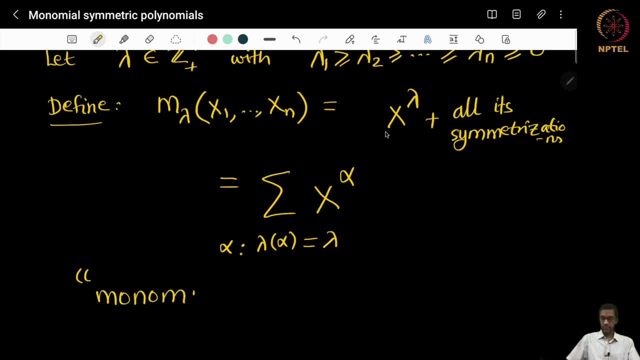 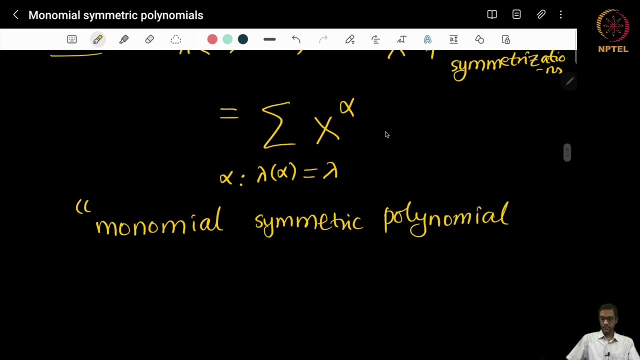 with symmetric polynomial, indexed by alpha, indexed by lambda And, of course, the two examples that we already talked about. so what are they? So if you take sample, you take three variables. so I take n equals 3.. And if I pick lambda? 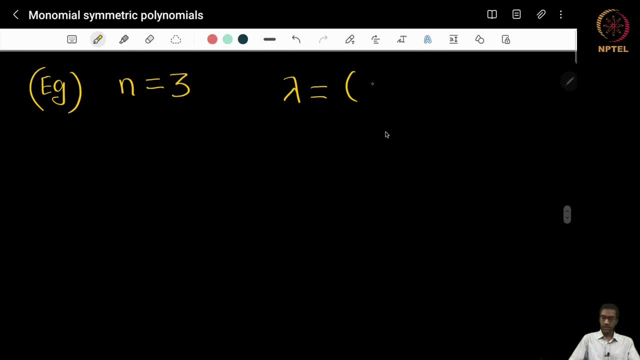 to be 3, 2, 1, then that is, the monomial symmetric function, is going to be sum of those six terms that we have seen already: x1, x2, x3,, 3,, 2, 1, plus 3, 2, 1, x2,, x3,, 3,, 2, 1, x1, x2,. 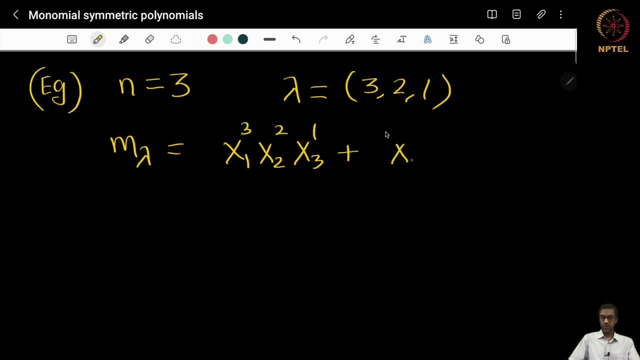 3,. in some other order, 3,, 1,, 2,, etc. So six terms total. So that is our usual example we have looked at previously. Now second example, if we take lambda, to be so same. 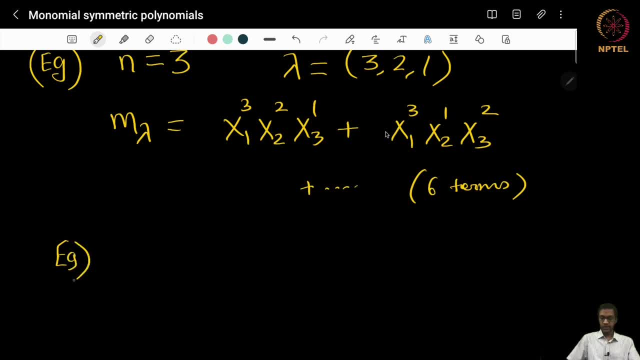 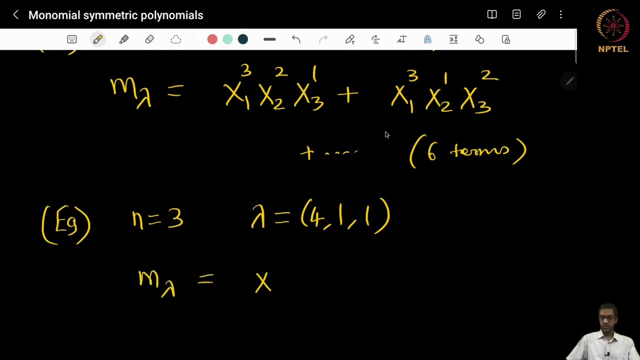 thing n equals 3, take lambda to be 4, 1,, 1, it is in weakly decreasing order. then M lambda, the monomial symmetric function, has the starting monomial just 4, 1,, 1, then. 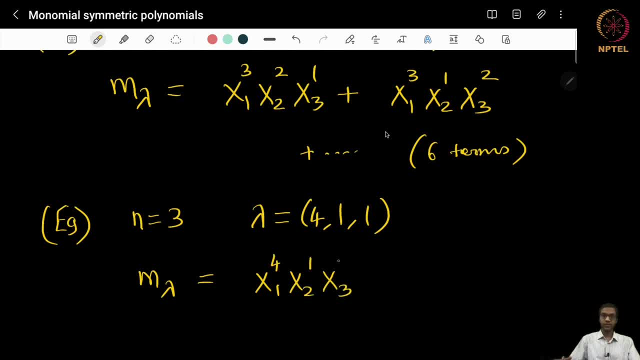 all the other alphas, such that when you arrange them in decreasing order, you get 4, 1, 1.. What are those? Those are exactly 1, 4, 1, and 1, 1, 4.. 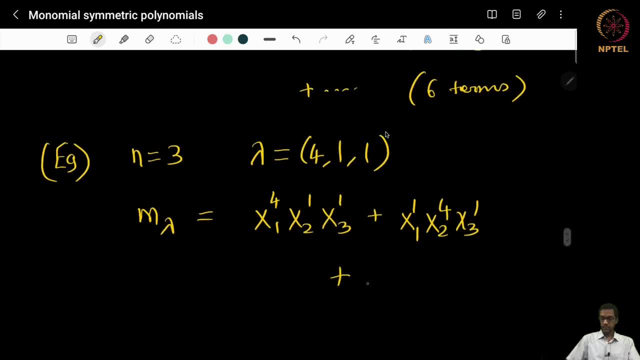 165.. mark lambda and 4 of l 176.. mark lambda: un"4ilescom문âu剛剛 открытр-. So that is the. those are the two examples that we already looked at. 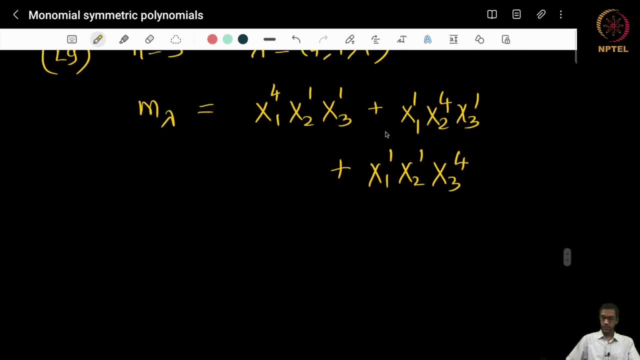 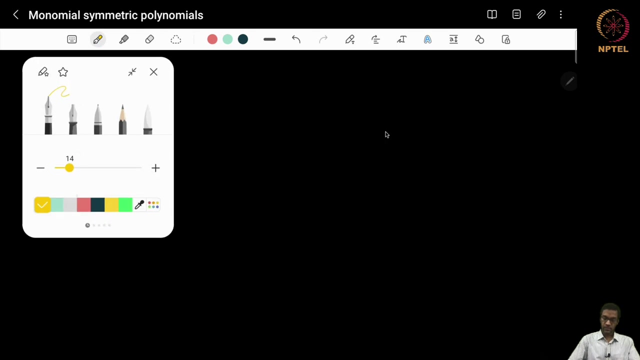 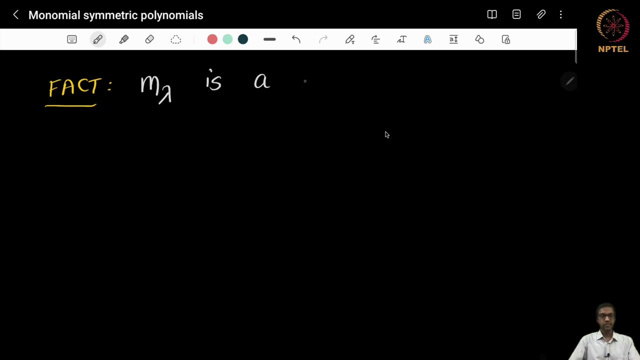 Now some quick facts about these symmetric functions, which is very easy to see. So observe fact: what is the degree of this monomial? so well, I should say the monomial symmetric polynomial m lambda. m lambda is well, its symmetric is clear, but more than 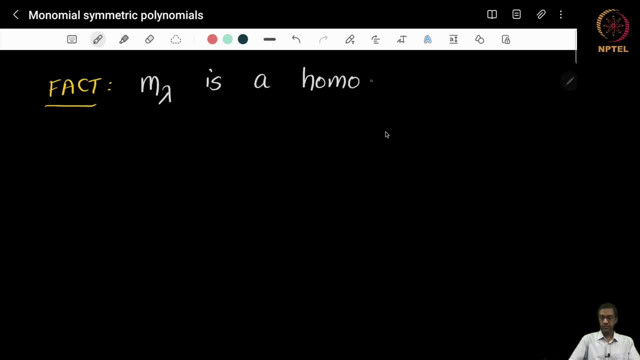 that all the terms which occur in it are of the same degree. So that is what you call a homogeneous symmetric polynomial. with a homogenous symmetric polynomial, What is the degree of all the monomials which occur in it? Degree of m lambda is exactly. well, as we have just seen the powers that go on top. 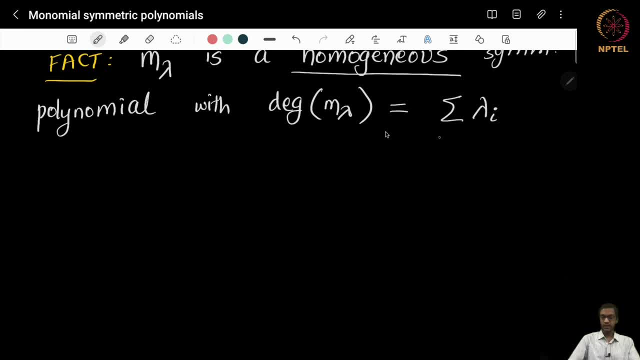 of the variables are just the lambda i's, And in every monomial you just get the same lambda i's, but maybe in some other order. But the total degree is just going to be the sum of all the lambda i's. So that is a simple fact. good. 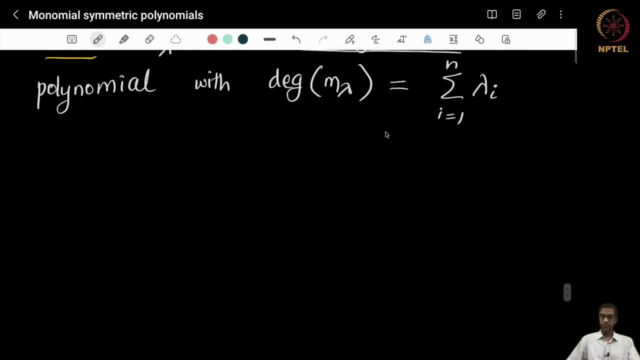 So let us, to sum up, To say a bit more about this. we just need some notation. So let me just introduce something which will come up again and again when talking about symmetric polynomials. This is what we call integer partitions, sometimes just called partitions. if it is clear that, 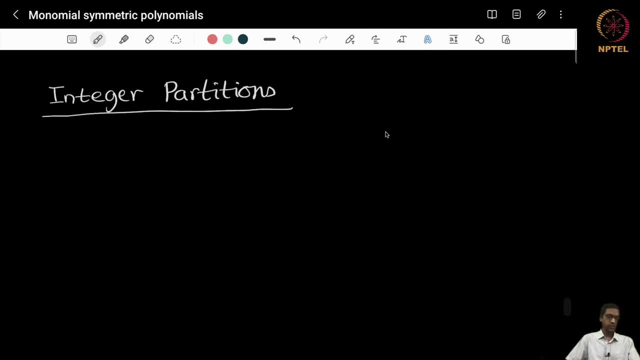 we are dealing with integers. So what is a partition? Well, it is definition. An integer partition or a partition is a decreasing sequence is well, what is it? it is a weakly decreasing sequence. It is something of the following kind: 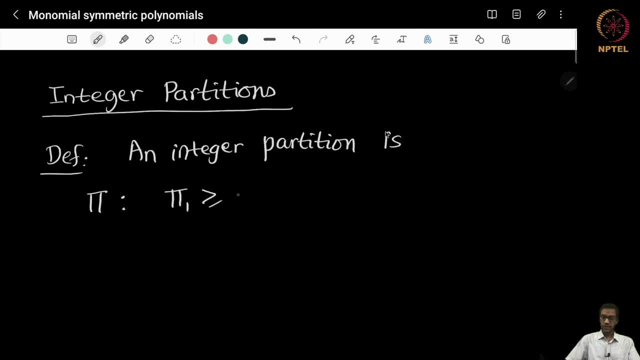 Pi is a decreasing, weakly decreasing sequence: pi 1, pi 2, pi k, And we assume that They are all positive, So they are all natural numbers now. So what an integer partition is? well, in words, it is nothing but a weakly decreasing. 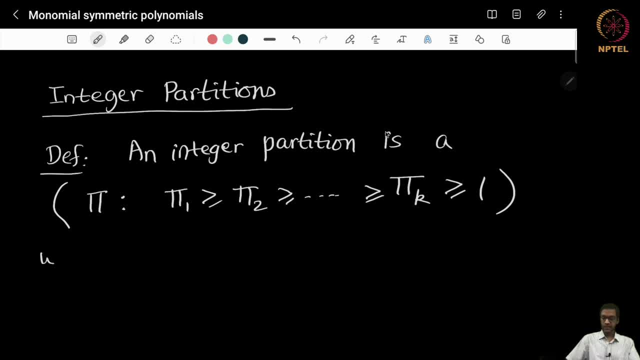 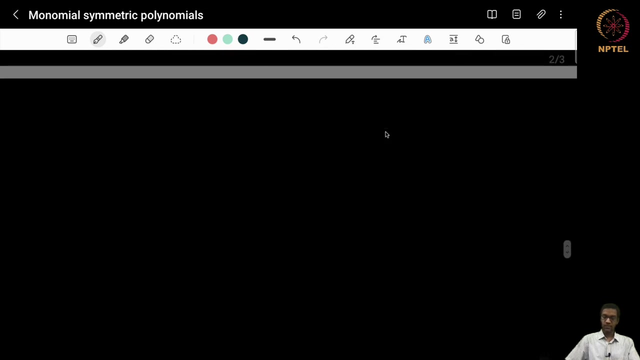 sequence. So this notation is a weakly decreasing sequence of natural numbers, And this is usually how we write it. We call it pi and then we write pi 1, pi 2, pi k- Exactly. Sorry, This is not after the beginning of the session, when we Righteous and cyclic sen清. 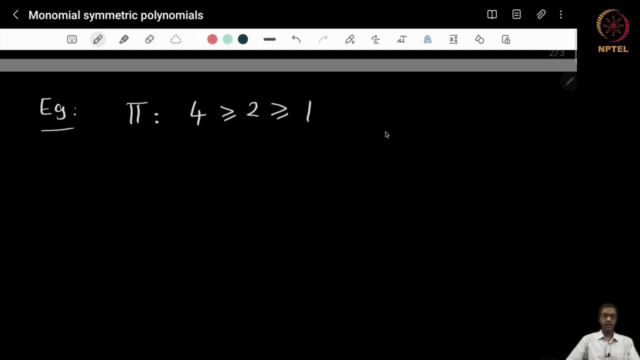 in our problem. ceaseless fact жизни. simple, it is some iterations and simple properties. So well, examples. first example, for example, 421.. This is you can think of the tuple 421 as a partition, or you can look at, say, 211, that 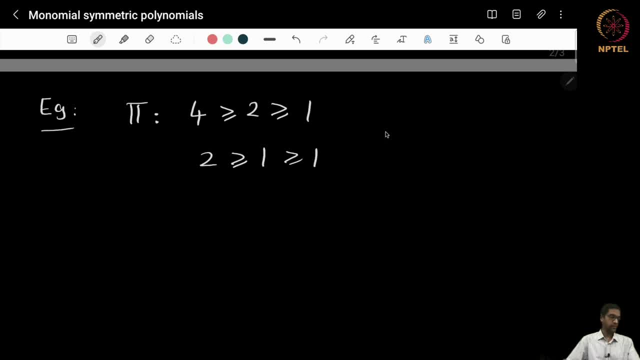 is also partition, And so these are all examples of integer partitions. Now we have some standard terminals. Can I bring you a bit size Right? We have some articles. Let us not speak, won't we terminologies or notations. here we write, given a partition pi, we write mod pi to be the sum of 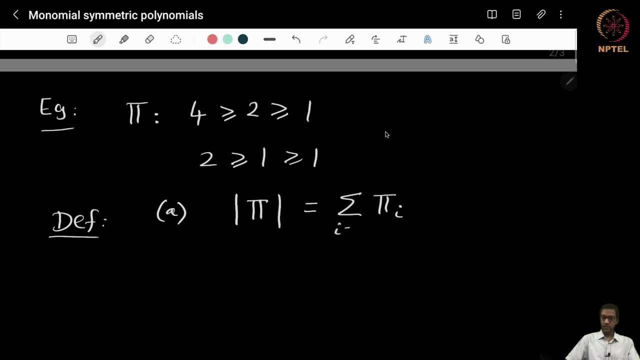 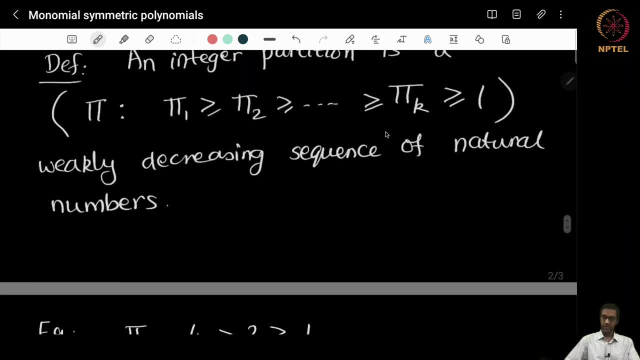 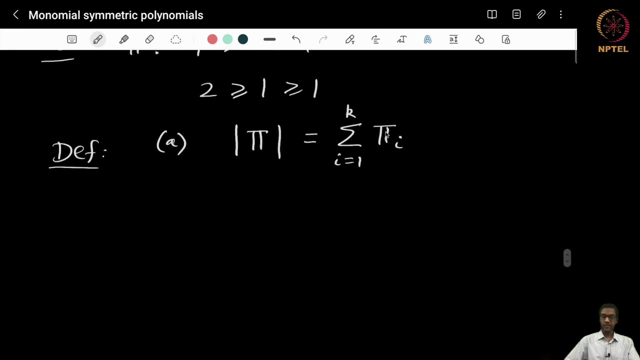 all the pi. i's okay. so i said there are k parts. okay. so what is what is k here? k is in, as in my original definition here, so i wrote pi as pi 1, pi, 2, pi, k. so there are k natural numbers arranged in decreasing order. mod pi is just a sum of all those natural numbers. okay, and length of pi. 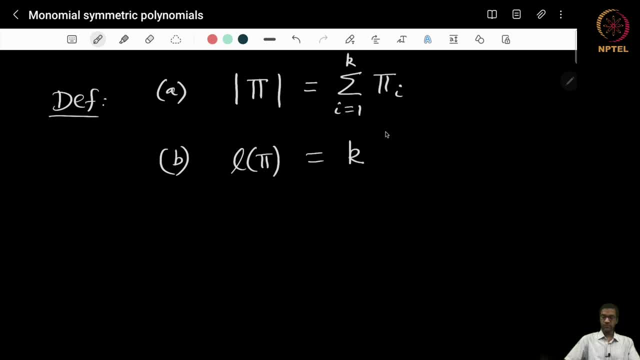 is the number of elements of the sequence, so it is that number k. okay, now we also tend to think of, you know, partitions, when we write a partition as pi 1 greater than or equal to pi 2, and so on. but we often think of pi really as follows: so pi is thought of as: 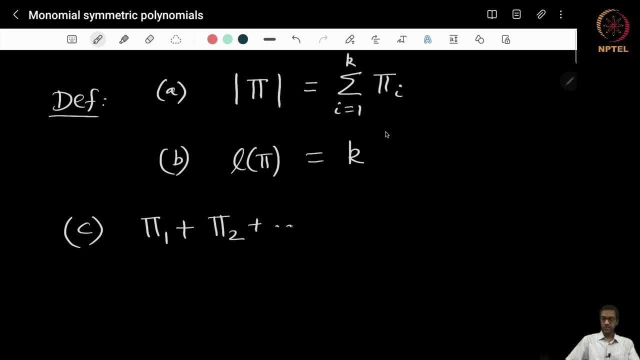 really the sum. see, this is how we really think of of an integer partition. it's pi 1 plus pi 2 plus pi k. so example, so you know. so so what is this? so here's an example. just come back to this. so 4 2- 1 that we wrote out already. we think of this as being the, the partition, or the, the sum: 4 plus. 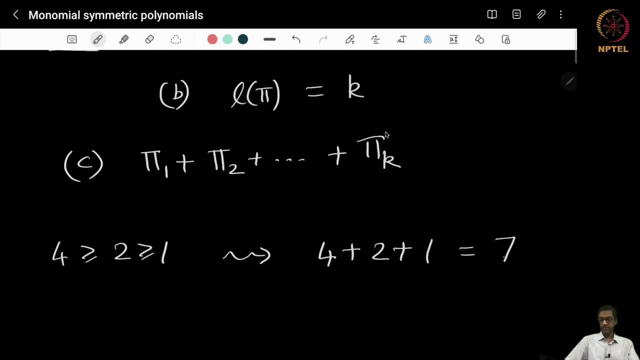 2 plus 1. okay, and observe: 4 plus 2 plus 1 is 7. so what is this? 4 2 1 telling you it's a way of splitting 7 into a sum of natural numbers. okay, and we don't want to keep you know, we don't want to think of 4 plus. 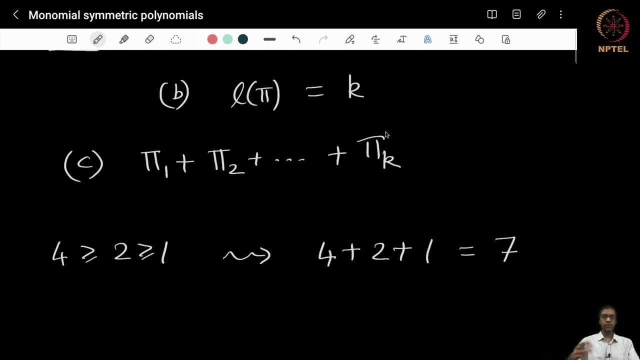 2 plus 1 as being different from 2 plus 4 plus 1, or 1 plus 4 plus 2, and so on. so we just want one single way of of saying: okay, i've taken 7 and i have sort of split it into these three numbers. 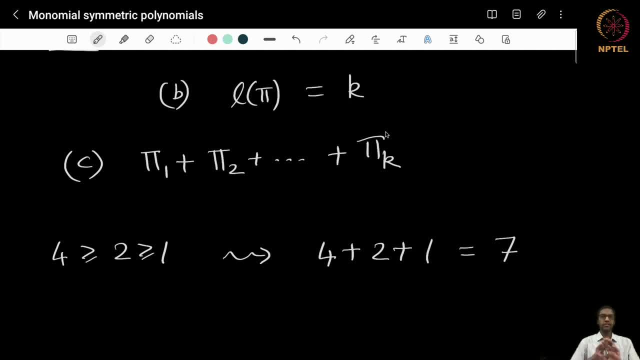 4, 2 and 1, and so we we just say, okay, let's just arrange it in decreasing order so that we don't keep counting the same thing, think of the same thing in different orders. okay, so 4, 2, 1 is is a. 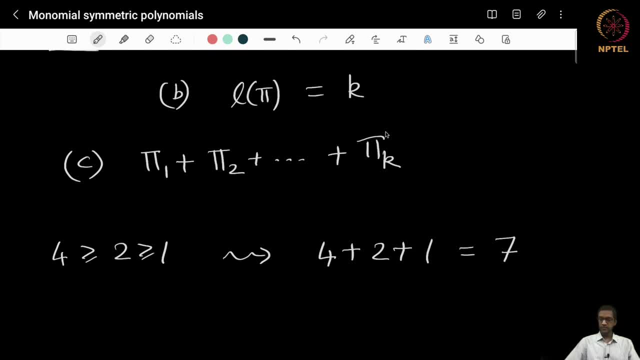 partition of 7 and the well, the, the, the individual elements, pi 1, pi 2, pi k are sometimes called the parts of the partition. okay now, so this is usually how we are thinking of a partition as really being the sum. okay now, what else is? what else is important here? well, let's give these, these things, names. 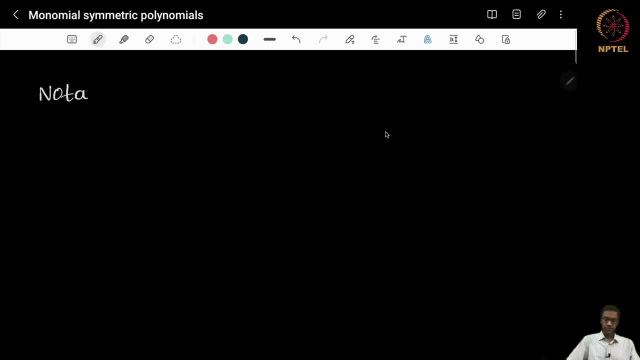 so here's some more notation: p of d script. p of d is just the set of all partitions of d. okay, this is the set of all integer partitions pi, such that mod pi equals d. okay, so we should. we say these are all partitions of d. okay, now that's one. here's another piece of notation. if pi, 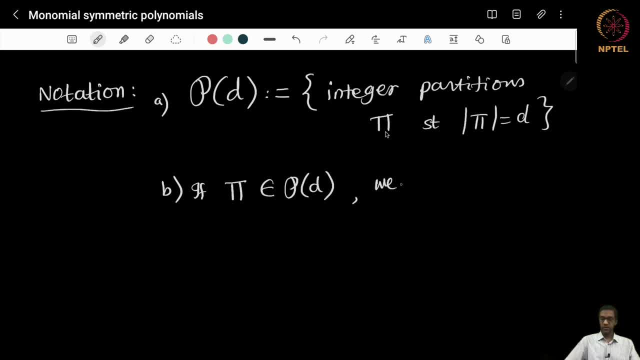 if mod pi is d, if pi belongs to pd. we also write so many different notations to express the same thing. we say pi and put the symbol here to say pi is a partition of d. this is how we read that, that funny symbol in the middle. okay, so this is another symbol and 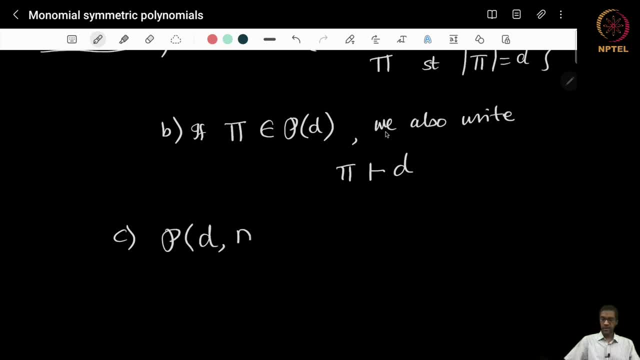 we'll also need to bring in n somehow. okay, and remember, for what we have done so far is the number of variables. so what is pdn? okay? so here d and n are natural numbers. so let's say d and n are greater than or equal to one. right then what's pdn? well, this is the set of all partitions. 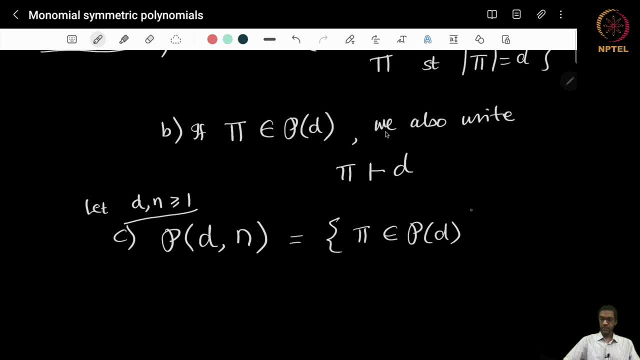 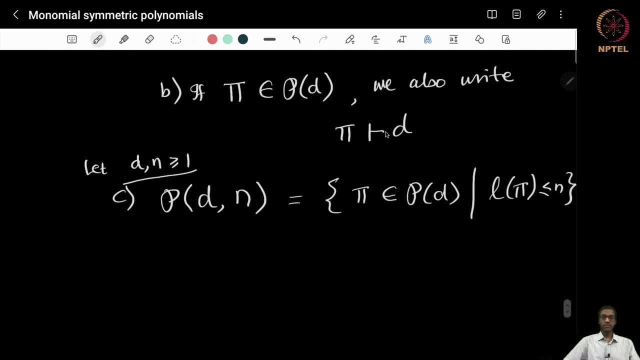 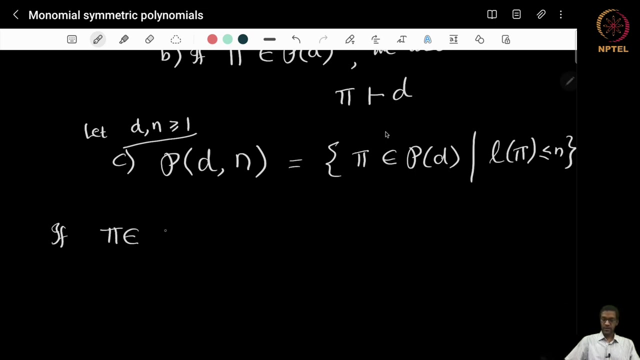 of d, such that the length is at most n, which means recall. the length is just the number of parts, the number of natural numbers that occur in the sequence pi. okay, now if you have an element in pdn, so if pi belongs to pdn, what does it mean? it means pi. 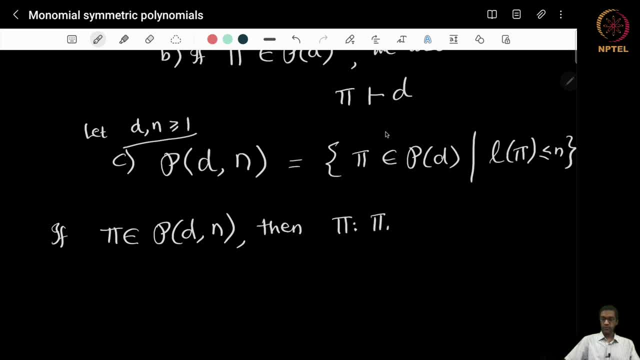 can be written as follows: pi 1, pi 2, pi k greater than or equal to one. with k is a number of parts right, that's the length k is supposed to be at most n. that's the definition. okay, so you have less than n non-zero numbers. pi 1 by 2, pi k here. 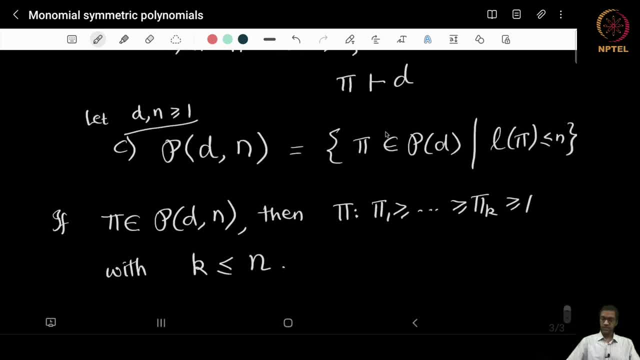 but in practice what we'll do is we'll often think of this. so i mean, here's one thing you can do: you can think of this as a sequence which is n times n times pi minus 1, pi, 2, pi k, and then we can write. 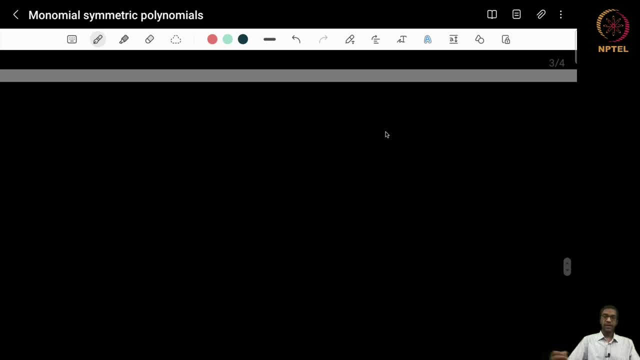 sequence with exactly n numbers by appending some zeros at the end. So we can also do the following: we can append well, how many zeros- n minus k zeros- at the end and think of pi as a sequence with n numbers as pi 1,, pi 2, pi k, and then we just put zeros for. 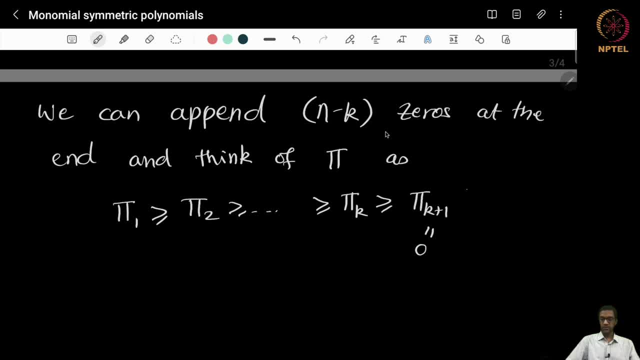 all the rest, just define this to be 0, 0, 0.. So now it is exactly an n-tuple of non numbers. So now it is exactly an n-tuple of non numbers. So now it is exactly an n-tuple of weekly decreasing numbers. Now, why are we doing? 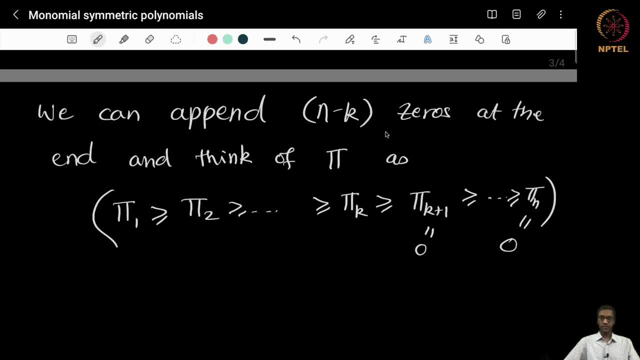 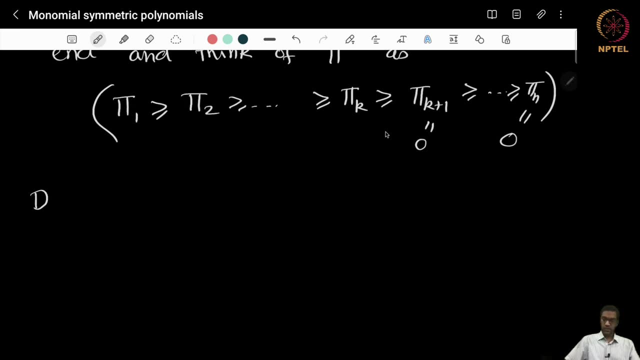 all this? Well, because, of course, we are interested in talking about monomial symmetric functions, where these n-tuples of weekly decreasing numbers are what you need to index the monomial symmetric function. So now, why am I doing all this Recall? maybe not recall? let us 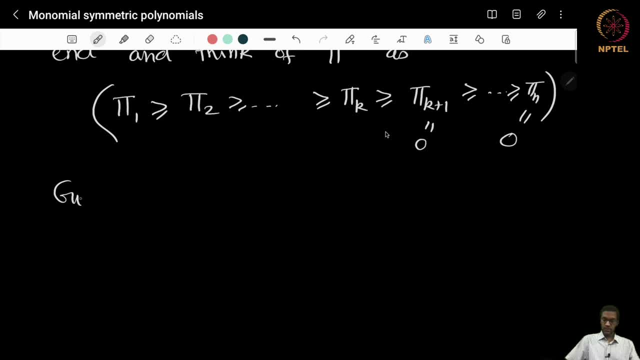 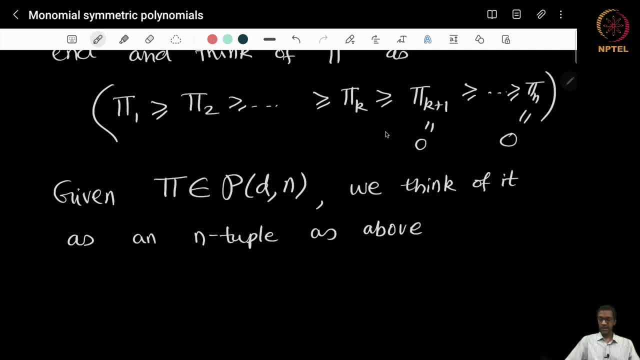 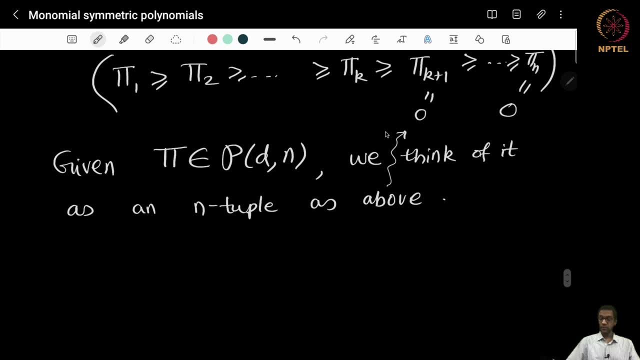 n-tuple at the end. So what we will do is to say we think of it as a partition pi, as above, as we just described by pending some zeros, And once you do that you can use that pi to index. So let us call this instead of pi. let us maybe call it lambda. 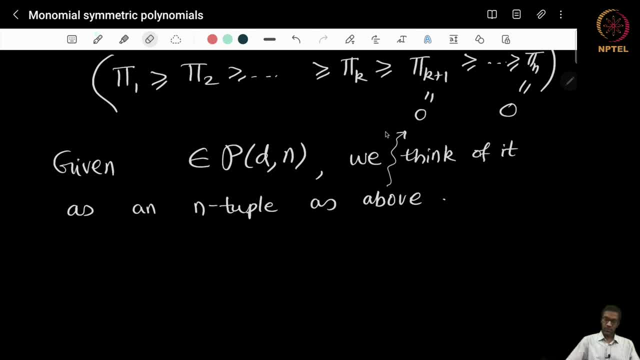 to be consistent with the lambda that we have been using throughout. So, given an n-tuple lambda, given a partition lambda of D with at most n parts, we append n minus k zeros and make it into exactly n numbers which are weakly decreasing, Then define, then look. 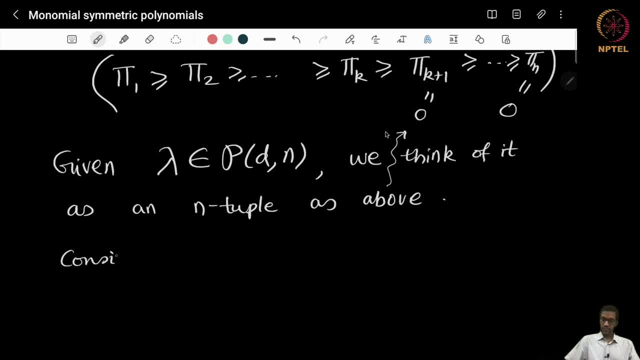 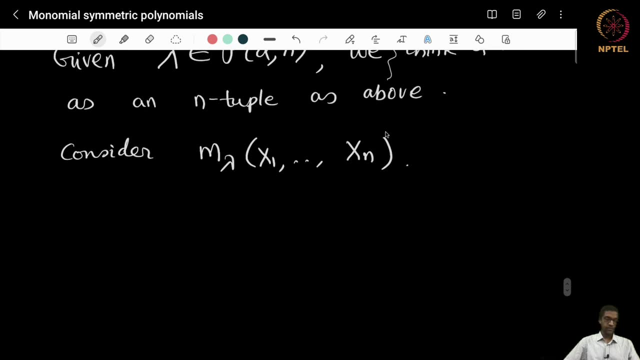 at, then consider the corresponding monomial symmetric function. So this is what we are going to do: We are going to take all such partitions in PDN and look at the corresponding m lambdas. And here is the key theorem. This may be the first important theorem that we 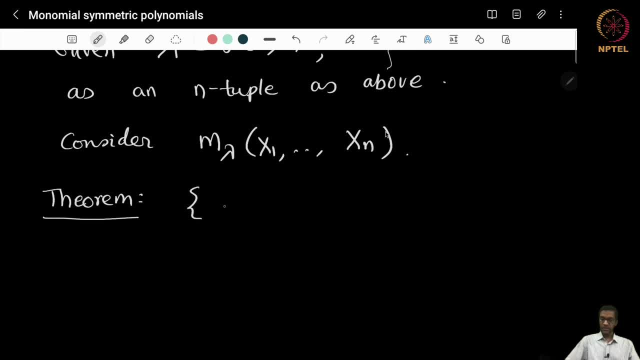 will encounter in this business, which is that these monomial symmetric functions, the m lambda, x1, x2, xn, when lambda varies over the partitions of D, with that most n non-zero parts. This set- and you know the meaning- is what we have said above: you have to append zeros to make. 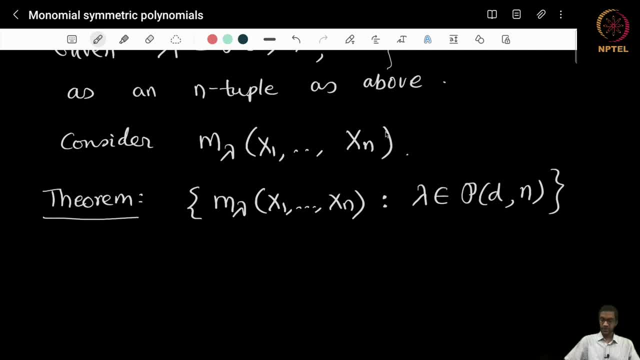 it exactly n-tuple. This collection of monomial symmetric functions is, in fact, it is a basis, But remember we were talking about, you know, everything was over z. we were talking about polynomials with coefficients in z. So this is a z basis of the space, of you know, the. 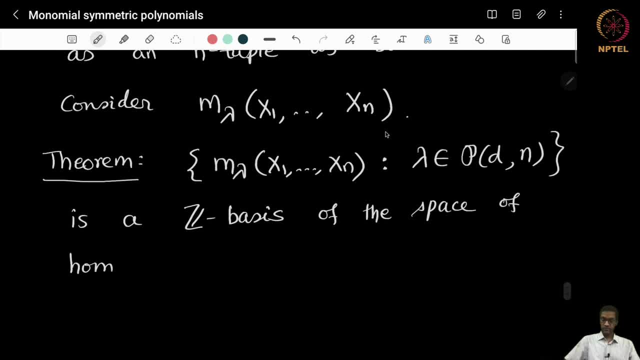 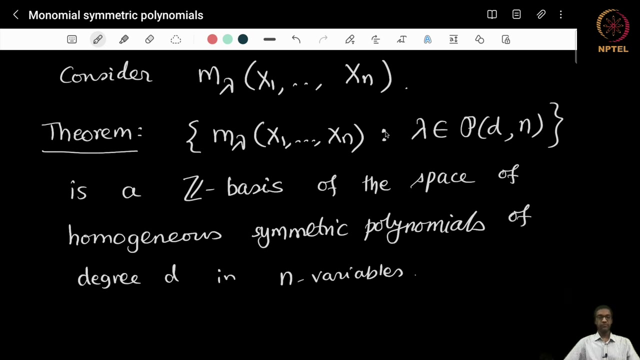 traverse. So we need the homogeneous symmetric polynomials of degree D in n variables. The second one, The last one, The third one, Yes Now. so I mean if instead of z, we were talking about polynomials over, let us say, the Russian. 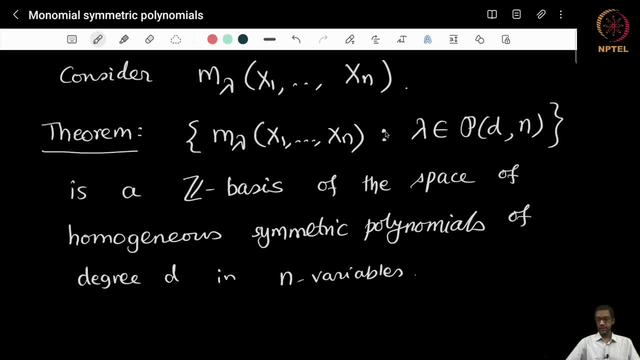 numbers or the complex numbers or other fields, then this space would be a vector space. And what we are constructing, what we are claiming here, is that m lambda would actually be a basis of that vector space. Now, here we are, working over the ring z, So maybe the correct 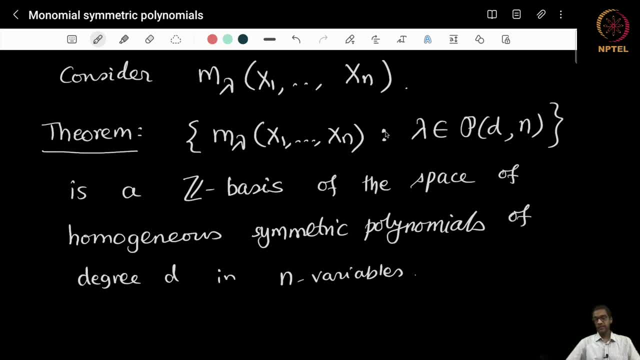 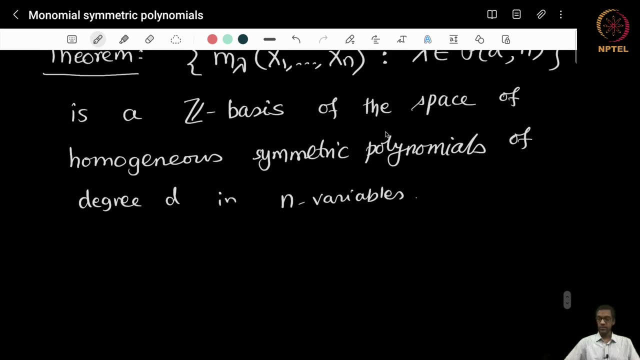 way of saying it is: it is a module over z and that this is this, forms a basis over that, over that ring R. Now, without really getting into too much of the technicalities of modules and so on, what we really need to prove in order to establish this theorem, 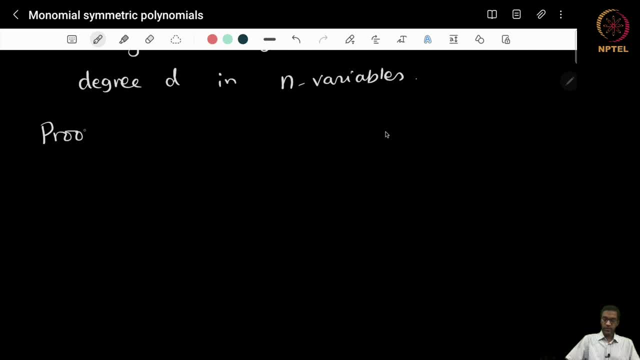 is sort of what the word basis usually means, which is that it is every element of every polynomial, homogeneous, symmetric polynomial of degree d in the variables x 1, x 2, x n. we need to show it can be written as a z linear combination of these m lambdas. 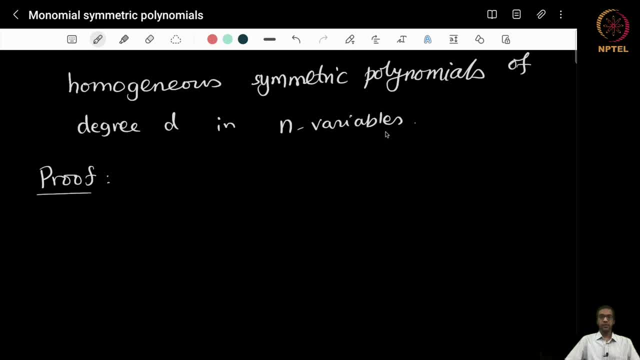 And secondly that so that is the spanning condition and the linear independence condition says that if some linear combination of the m lambdas gives you 0,, then the, the independent individual coefficients in that linear combination, have all got to be 0, the usual two properties. 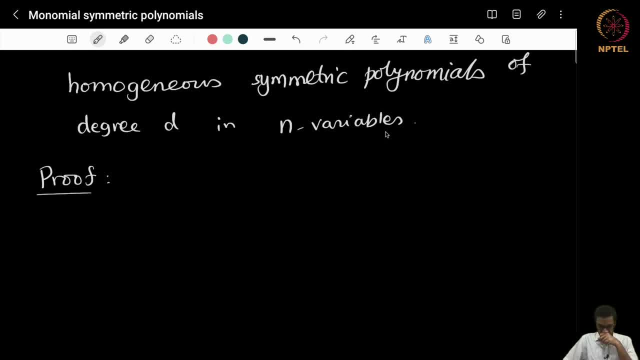 So let us, let us prove the first one, the spanning property. So let us take a polynomial that F of x, 1, x 2, x n be a homogeneous, symmetric polynomial of degree t. And what is the standard way of representing? 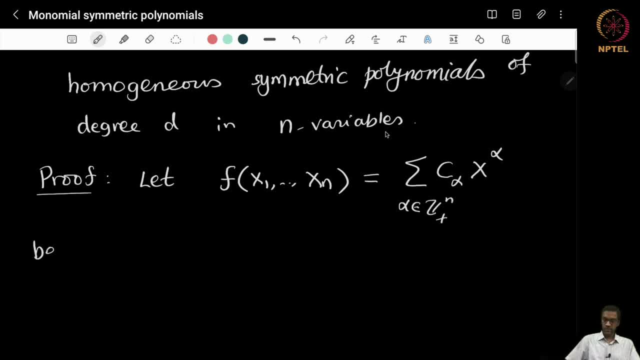 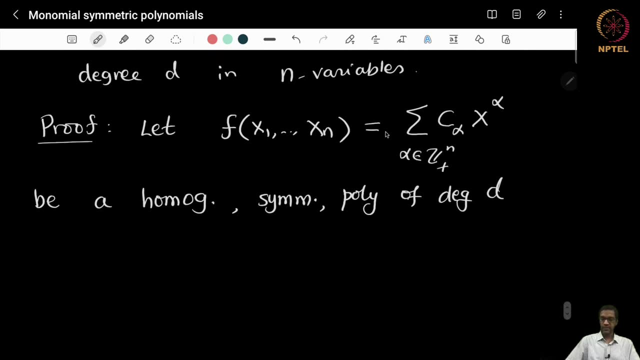 a polynomial- it is a sum of monomials- be a homogeneous, symmetric polynomial of degree t. Now, what does homogeneous symmetric mean? It just means that every monomial has the same degree. So what this means is that. so what we have is the following. So if you 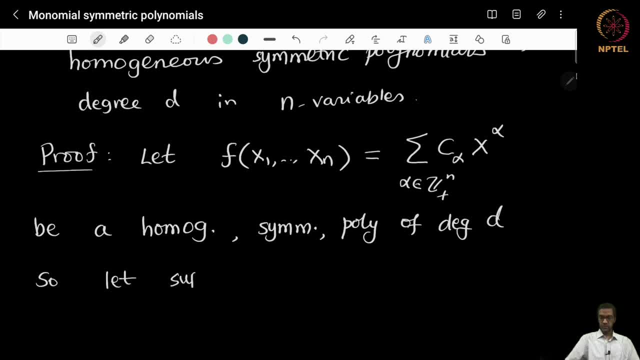 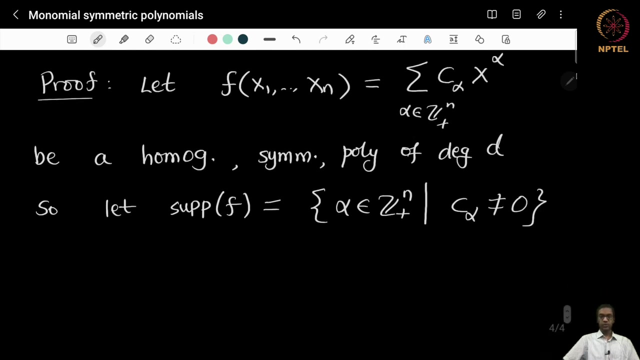 take. so let us call this the support of this polynomial. it is just those alphas. So just take the collection of alphas for which this coefficient is not 0. Now just take those monomials which actually appear. that is what this means. So let letting 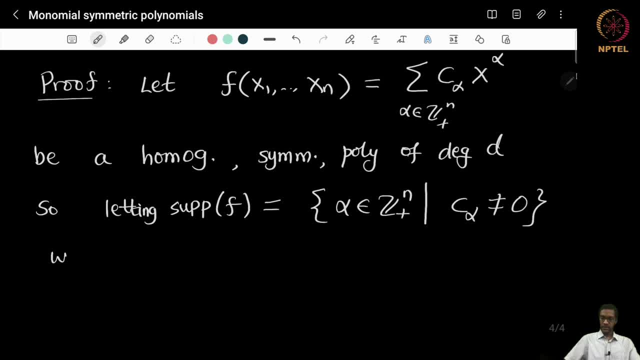 support denote this. we conclude that for every alpha in the support the degree is d of that corresponding monomial. So that just means the sum of the alpha i's must be d for all alpha in the support, The support of f. So that is just homogeneous of degree d. that is all it is saying Now. 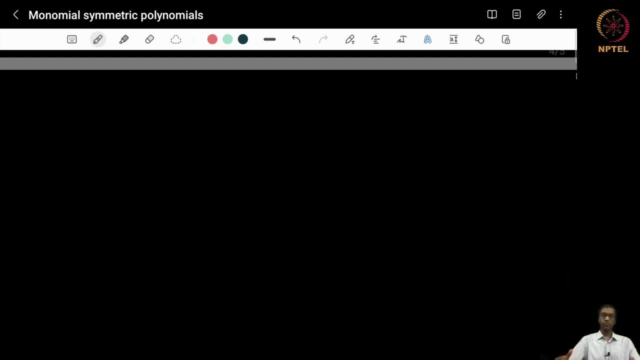 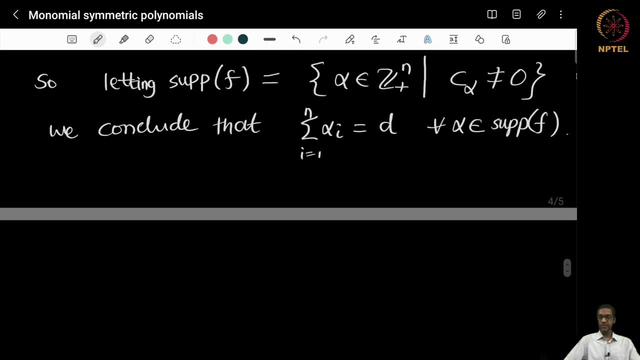 let us see how do you express this. finally, as a linear combination of monomial symmetric functions. Well, from each of these monomials, whose total degree is d, sum is d, we just pick out the ones which are in decreasing order, as we saw earlier. So let us call that. 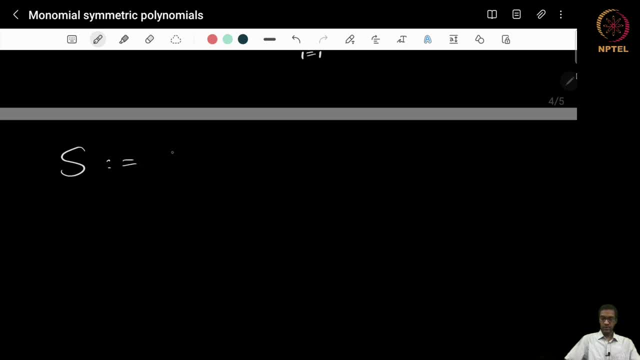 Let us set something, let us s denote the set alpha in support of f, those alphas which appear such that alpha is in decreasing order, alpha is weakly decreasing, And observe this is nothing but another way of saying this is support of f intersection. 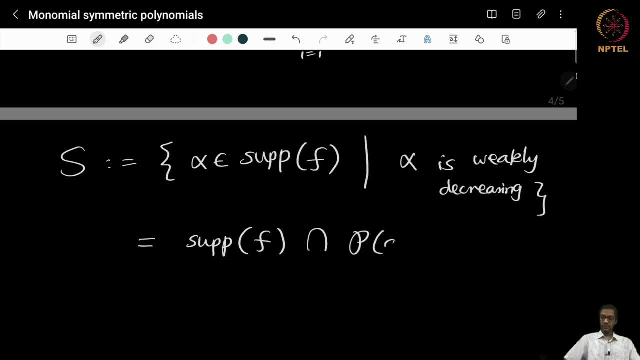 the set P d n. So P d n, recall, is just what: all numbers weakly decreasing numbers of length n with total sum equals d. So that is how we view partitions of the. as we said, the identification P d n is all those partitions with length at most n, but we think of them as having 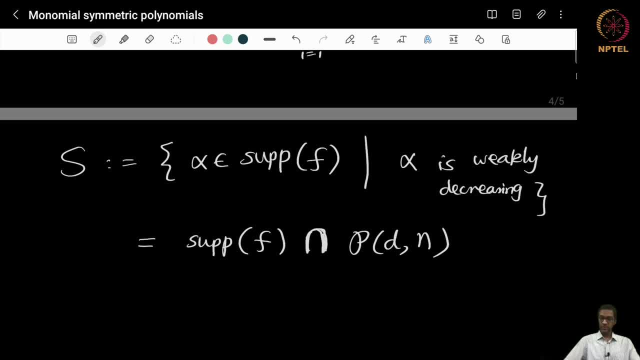 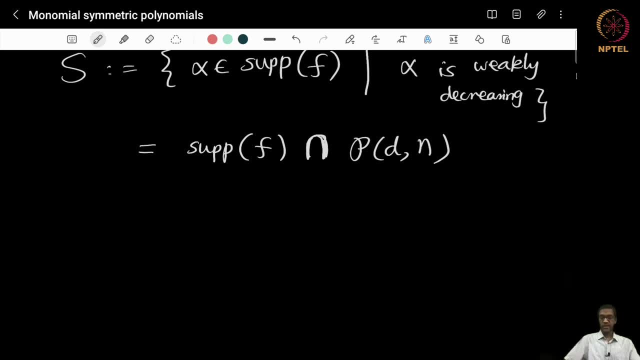 length, exactly n, by appending some zeros at the end. So this exactly. Now, the claim is that the fact that f is symmetric tells you something. it says that it is actually enough to just focus your attention on these monomials, whose exponents are in. 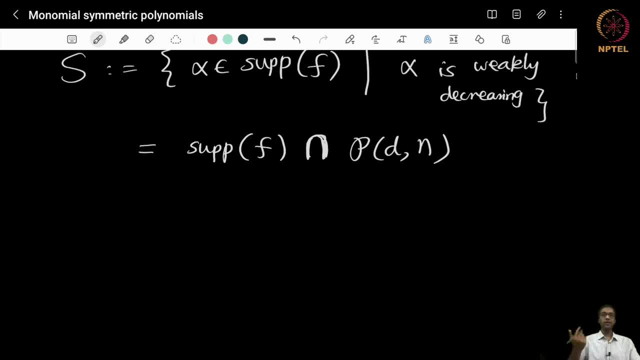 decreasing order, because that will tell you what the coefficients of all the other monomials are, because those are just obtained by permuting these indices. So observe: f is symmetric. So symmetric polynomial says that c alpha, the coefficient c alpha, will be the same as 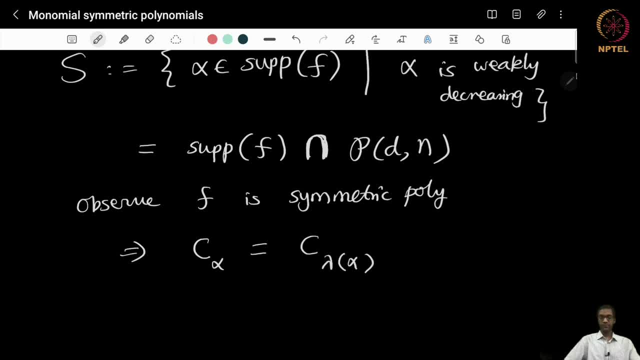 the coefficient of the monomial c of lambda of alpha. lambda alpha is the alpha arranged in decreasing order. this is for all alpha. So what does it mean? This just means that for the polynomial f can just be the same. So what does it mean? 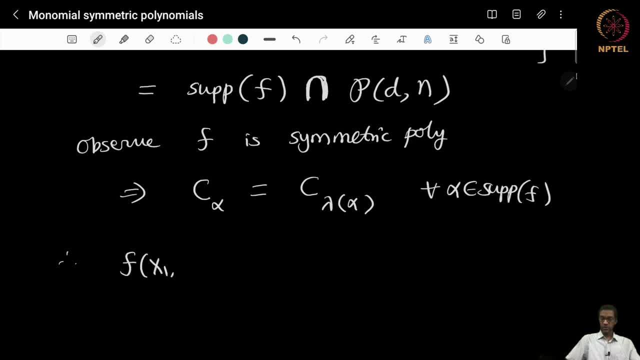 This just means that for the polynomial f can just be the same. So what does it mean? So it just means that for the polynomial f can just be written as follows: Instead of summing over all the you know, see earlier it was actually a sum over. 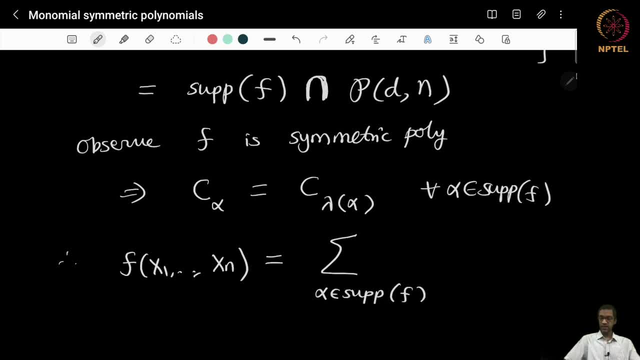 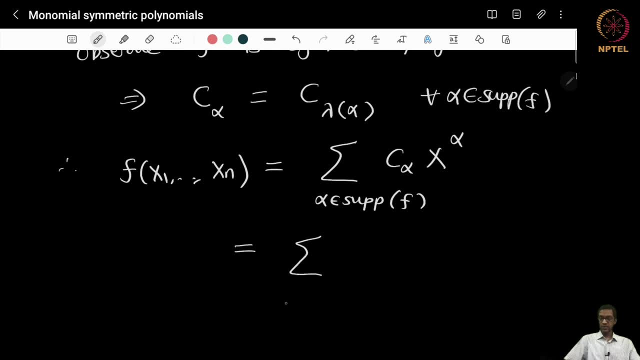 all alphas in the support of f, c, alpha, x, alpha. that was the original expression. But now what we are saying is: you just focus on those alphas which are in decreasing order. So I will just focus on those. I, instead of alpha, I will call it lambda. lambda as which. 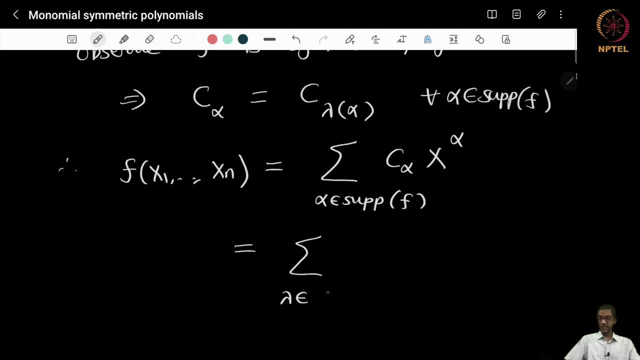 are in support of f, intersection p, dn, PDN, the ones which are in decreasing order. So that was what we call the set S. Now for this fixed lambda. what this property here says. what this property says is that the constant C alpha, 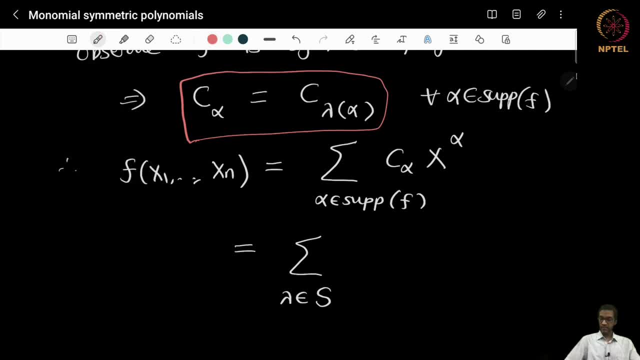 is the same as the constant C lambda of alpha. So I can pull out that C lambda term, constant from all the terms, And now this is just going to be some x alpha, where alpha is going to range over those elements of the support, such that the, if you arrange it in decreasing order, 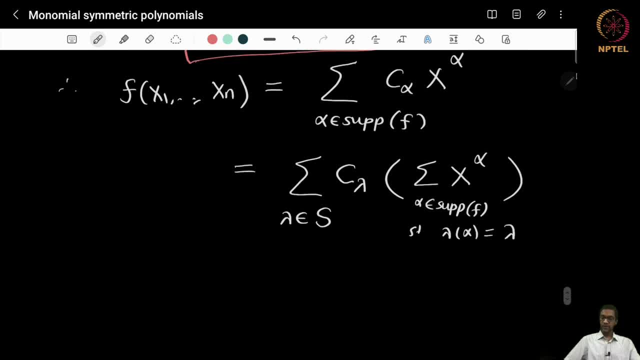 it gives you this particular lambda, And now that is exactly what we want, that is, the monomial symmetric function by definition. So this is C lambda, m lambda. Okay, so this establishes the first part, that any homogeneous symmetric polynomial of degree d 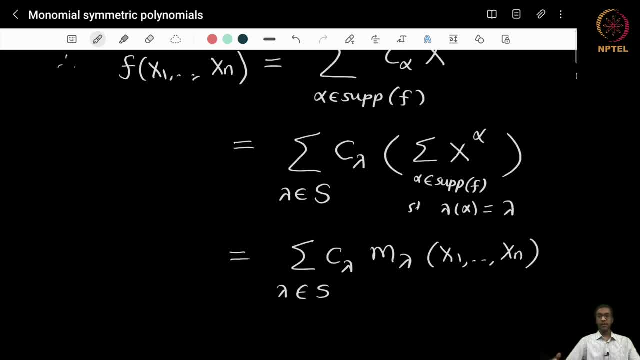 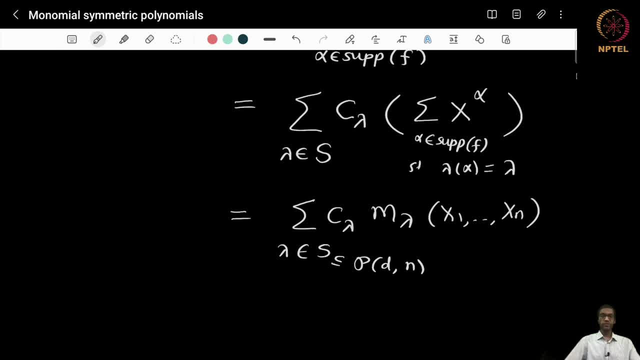 the given F as a linear combination of the m lambdas, where lambda varies over PDN. Okay, that is the first thing. Now, second statement we want to prove is that the linear independent statement? So what does in some sense, linear independence now? 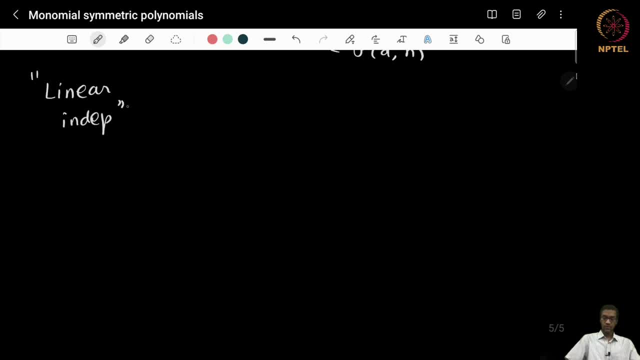 require. It says that if a certain linear combination is 0, lambda ranging over PDN, then each of those C lambdas must be 0. Now observe that. well, if you just stare hard at this left hand side, you will observe the following fact: that the 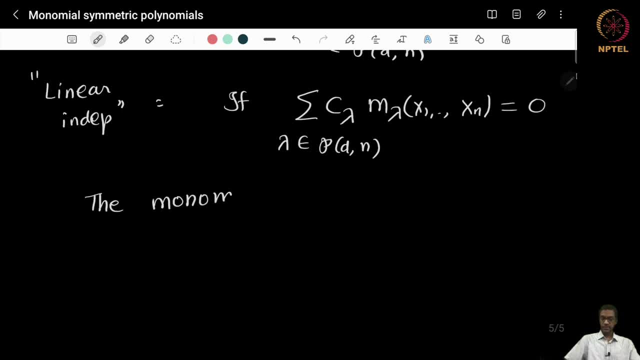 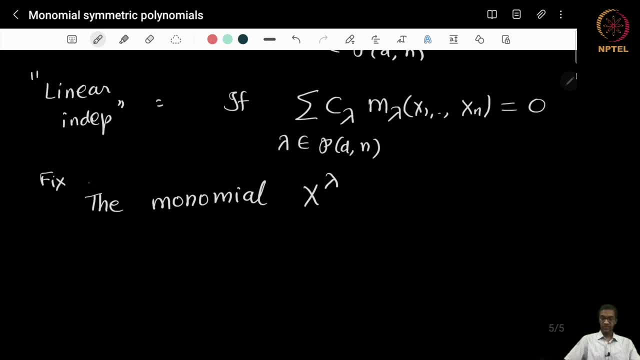 you fix a lambda, So you fix a lambda, So you fix a lambda. So maybe we should call it something else. Fix mu, maybe. in PDN, take a particular element and look at the coefficient of that particular monomial x to the mu. Now, what is the? you know, when does it? 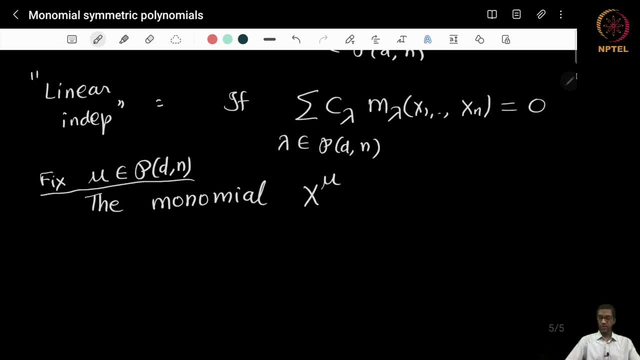 how can it possibly appear on this left hand side? the monomial x to the mu occurs on the the LHS only in the term m, mu of x1, x2, xn. There is no other way you can get the term. the monomial x power mu, mu is already in decreasing order for it to occur on the left.